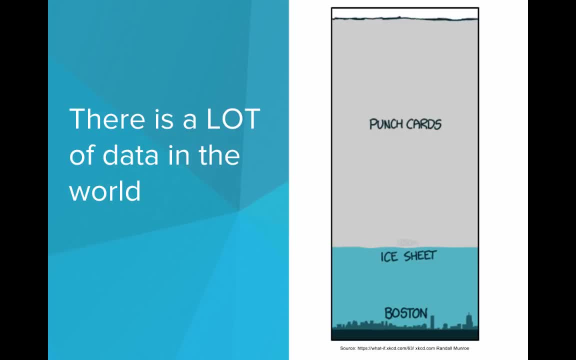 to put all of their data on punch cards. the amount of punch cards would be able to cover New England to the point that Boston would be buried significantly deeper than it was during the last ice age. Now, luckily, Google's not putting all their data on punch cards We have 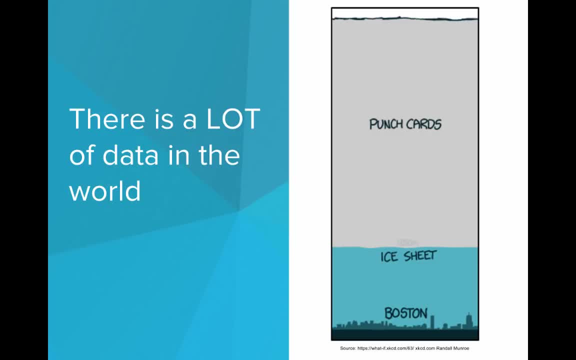 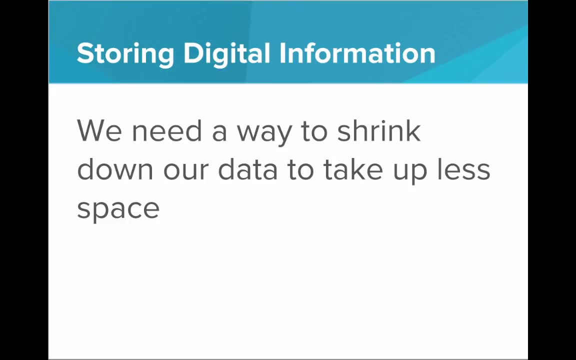 much more clever ways of storing data on hardware like disks and tapes and drives, but the hardware only goes so far. We really need a way to shrink down our digital information. We need a way to shrink down our data to take up less space. The hardware does a pretty good job, We're finding. 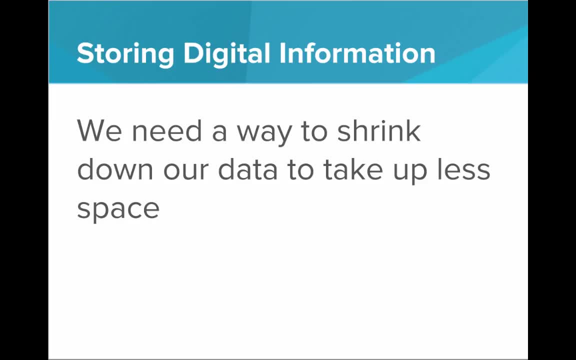 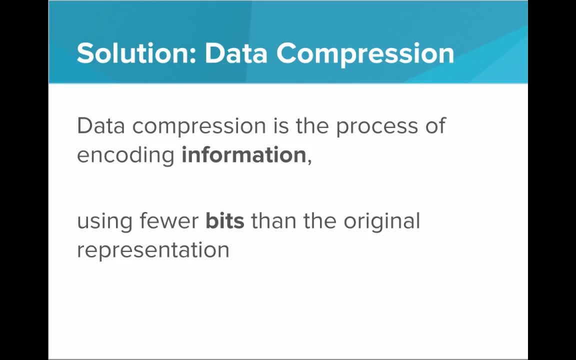 solution, And the solution here is data compression. So data compression is the process of encoding information using fewer bits than the original representation. So we've seen all of these ways to encode data using bits. We've seen the ASCII encoding for text. We've 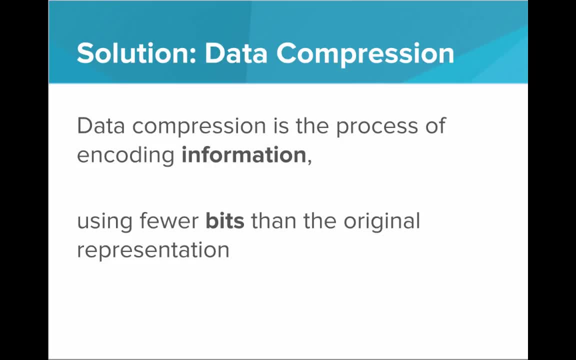 seen the RGB encoding scheme for colors and images. But these encoding schemes aren't really concerned with saving space, They aren't really concerned with using as few bits as possible. So what compression does is it takes this information and it takes the bits and it compresses them down to encode the same information using fewer bits than. 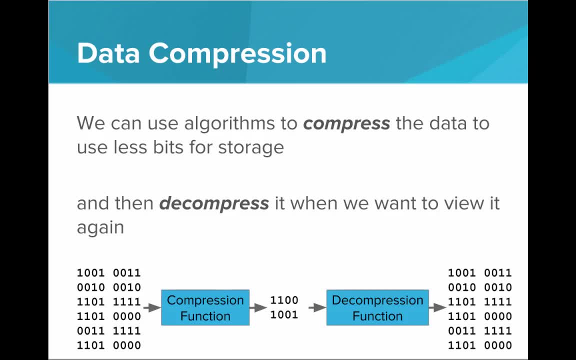 the original representation. So this is how compression generally works. When we want to store our data, we will pass our data into a compression algorithm, a compression function, and that will compress the data to use less bits for storage. Then, when we want to view, 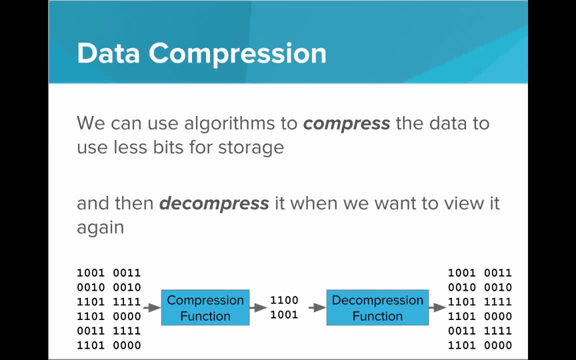 that data again when we want to see the image or see the text. we will pass that compressed data into a decompression algorithm And that will compress the data to use less bits for storage And that will decompress that data and restore it back to its original state. 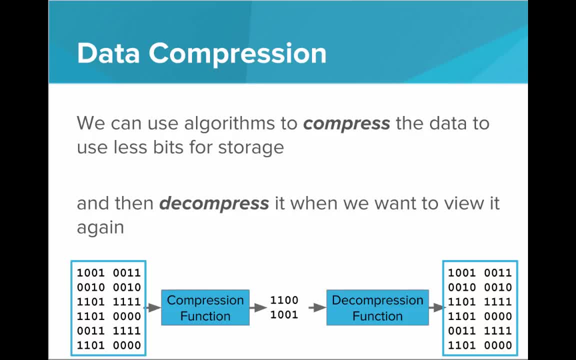 So we see here that the original and the decompressed data are exactly the same. So when this is the case, when we're able to fully restore the original data, this is known as lossless compression, And this is incredible. There's algorithms out there that can take data and 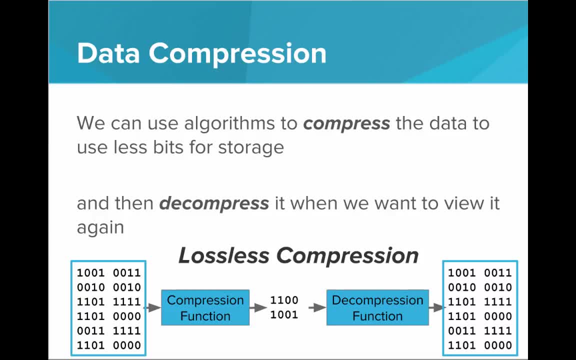 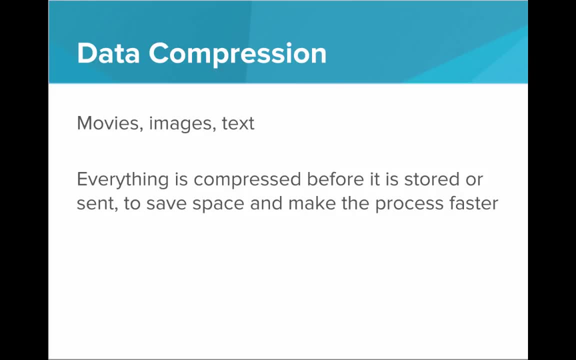 pack it down to almost half its original size and still recreate the original. It's really mind-blowing. So this is what we're doing every time you're interacting with digital information: Movies, images, text- all that information you're viewing on your computer is compressed before. 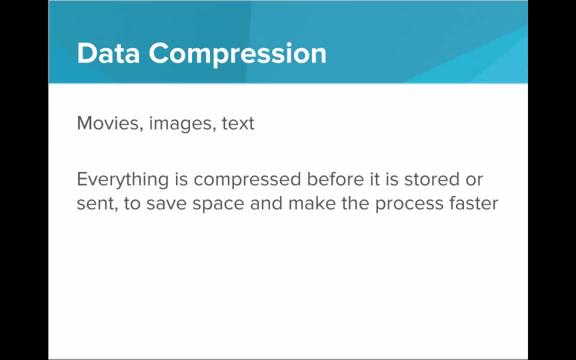 it is stored or before it's sent, And this is in order to save space and make the whole process faster. So why exactly do we compress data? Well, one is to save storage space. Like we've seen, we have way too much data. We need to come up with clever ways to store it. We're not. 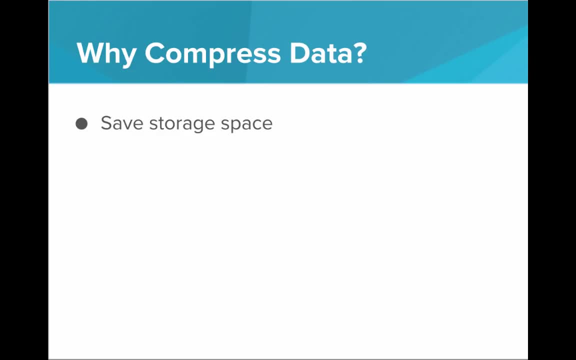 carrying around massive hard drives in our pockets. We have little phones, So we really need to use that storage space efficiently if we want to be able to access all of our data. But besides just storage, it also speeds up the time it takes to transmit data A network 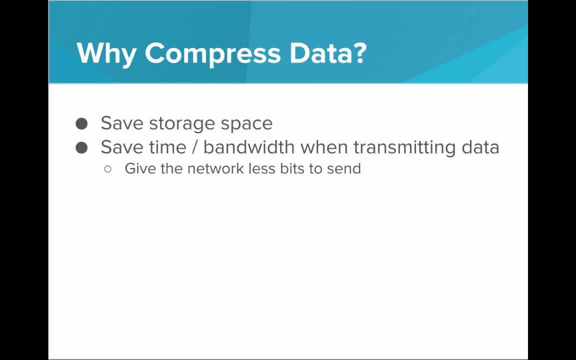 like the internet can only handle so much data at once. So if we compress our data before we send it, then we'll be able to send a lot more information over the internet And it'll take less time because we have less bits to send. 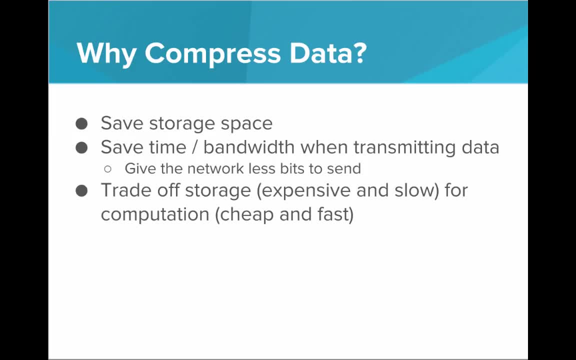 And at a high level. we're really trading off storage, which is expensive and slow, for computation which is cheap and fast. And what I mean by this is, in general, we're okay with using a lot of computation, But if we're able to send a lot of data, then 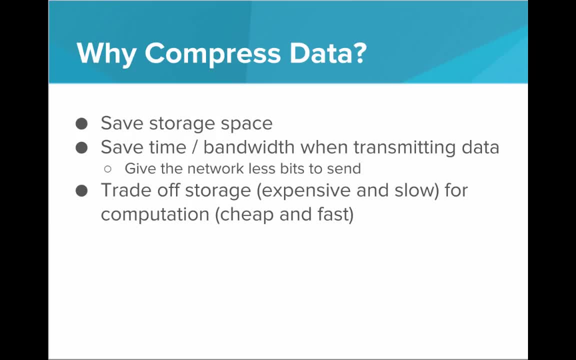 we're okay with using a lot of computation if it means that we don't have to use that much storage. Take your phone, for example. So your phone really doesn't have enough storage to carry around a 300GB raw movie file, for example, But if you want to carry that movie around, 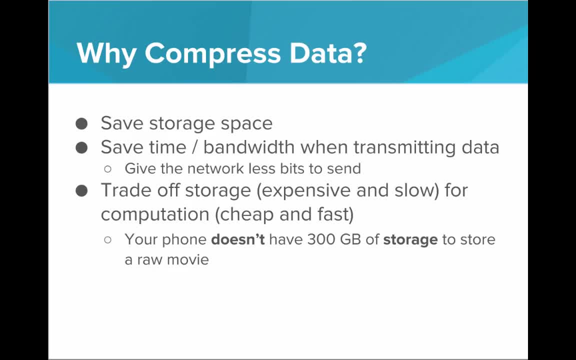 on your phone. what you can do is compress it down to a 1GB file. Then, when you want to watch the movie, your phone actually does have the computation power to decompress that 1GB file into a full movie. So we generally have a lot more computation power on our devices. 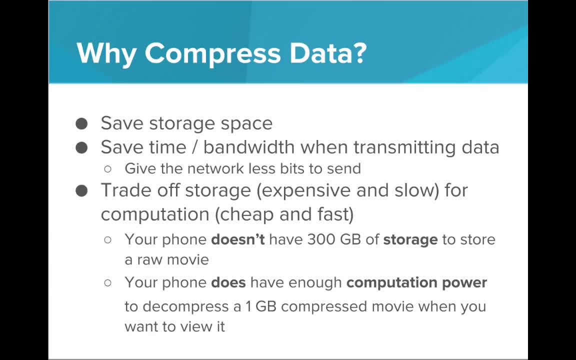 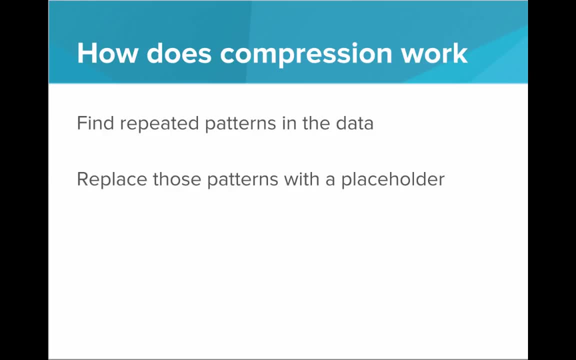 than we do storage, So we're trading off storage for computation. How exactly do these compression algorithms work? So, really, the way all compression works is we simply find repeated patterns in the data and we replace those patterns with a placeholder that is much smaller than the original data. For example, say we had an 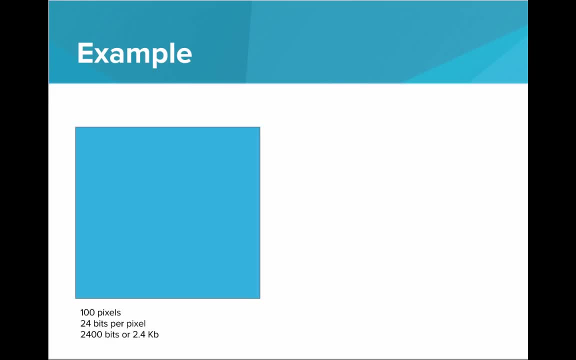 image. that was just a massive blue square. We have 100 pixels of blue. Well, that's 100 pixels and 24 bits per pixel- RGB, making it 2400 bits, But really the whole image is blue, so we don't really need to store every single pixel. 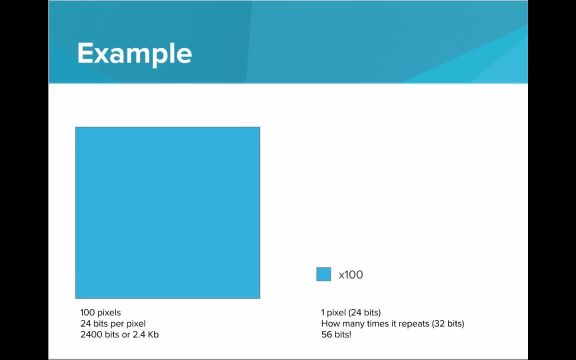 Instead, we can store one blue pixel and then also store the amount of times that it needs to be repeated. So here we have one pixel, that's 24 bits, and then we also store the number of times to repeat. 100 times, and that might be 32 bits. You put that together. 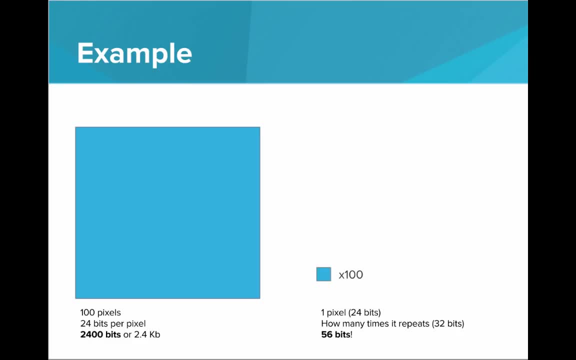 and you only have 56 bits. So we've compressed all that information- 2.4 kilobits- into 56 bits. Now this might seem like a silly example, because usually we have a lot more complex, but we're not going to do that. So we're going to do a little bit more complex and 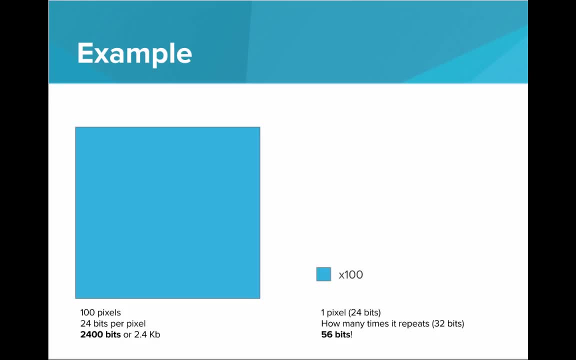 we're going to do a little bit more complex data than just a simple blue square, But you'd be surprised how much information is actually repeated in all of the images, movies and text that we use. Let's look at an example: compressing text. 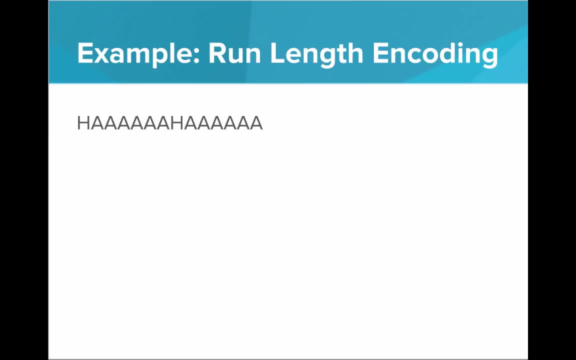 So one algorithm for compressing text is known as run-length encoding, And how this compression algorithm works is it takes each character in the original text and writes that character followed by a number of how many times that character is repeated to the compressed text. So, for example, here I have a single H, so I will write H1 to the compressed text and 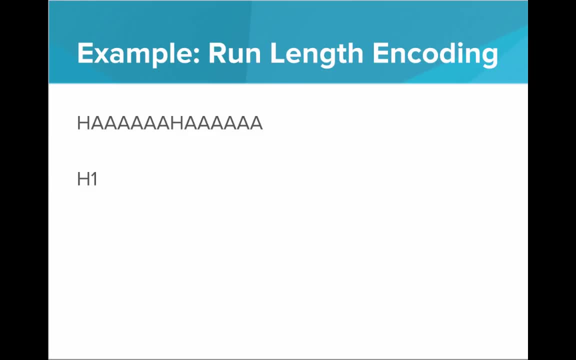 then I'm going to write H2 to the compressed text. So I have one H and that is followed by six As So, rather than typing out all those A's, I'll simply write an A and a 6 to the compressed file. Then we have another H again. 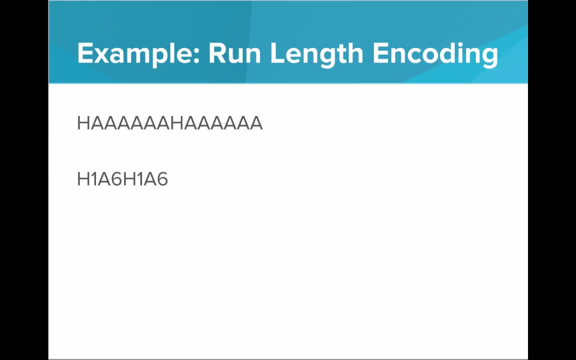 so H1, and then we have six more. As so, I'll write A6. And this is it. This is our compressed file, and it is much smaller than the original We see. in the original we have 14 characters, and since we have 8 bits per character, that's 112 bits. In the compressed version, we only 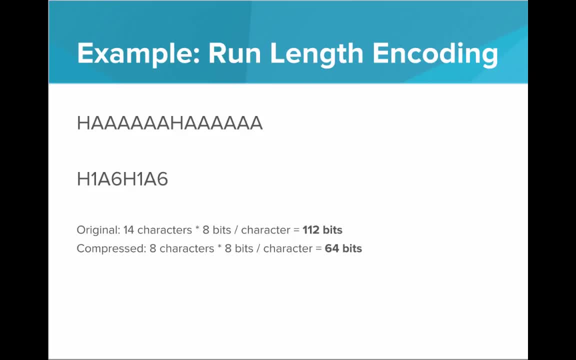 have 8 characters With 8 bits per character. that's 64 bits. Now, when we go to decompress, we need a decompression algorithm that reverses the process. So what we'll do is we will loop over the compressed version and we will write out that given character, that given number. 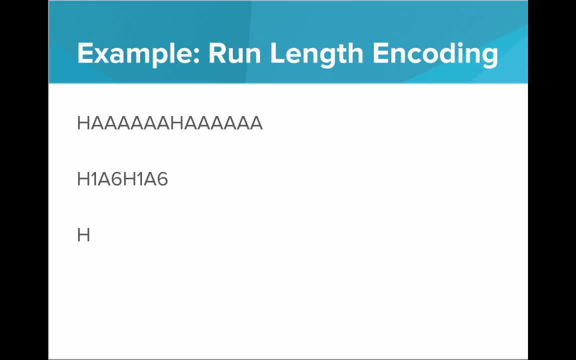 of times. So, first off, I see an H1, so to decompress, we'll write an H followed by an A6, so we'll write out six As, followed by another H1, that's a single H, followed by another A6, so we'll write out six more As, And we see that the decompressed version is. 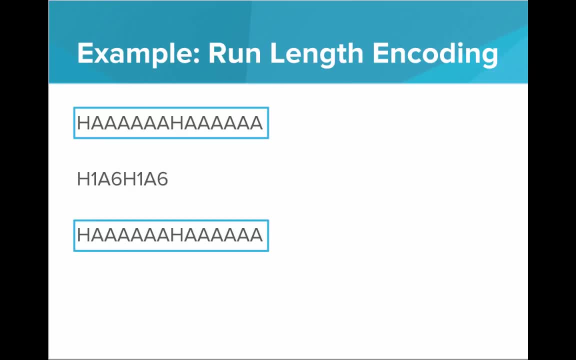 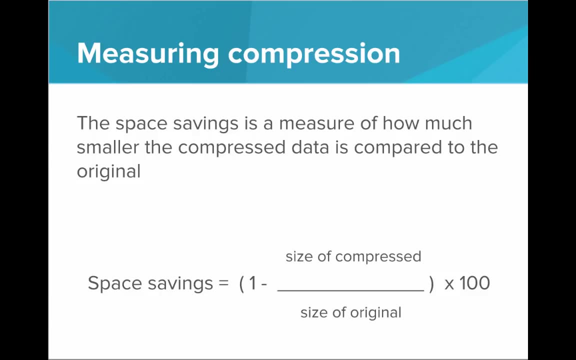 exactly the same as the original, So this was a lossless compression algorithm. Now, how do we measure a compression algorithm? How do we know when an algorithm is doing a good job? Well, one common measurement is space savings. So space savings is a measure. 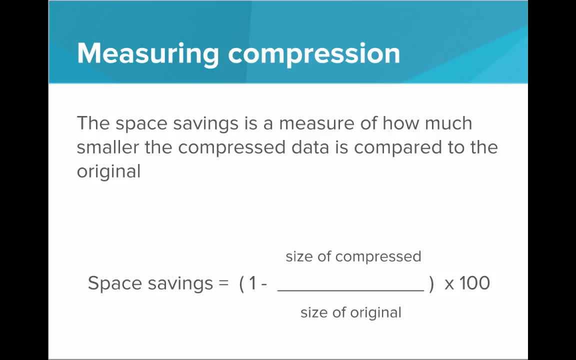 of how much smaller the compressed data is compared to the original. Now the formula for space savings is 1 minus the size of the compressed file, divided by the size of the original file, multiplied by 100. And what we get is a percentage of size decrease. So 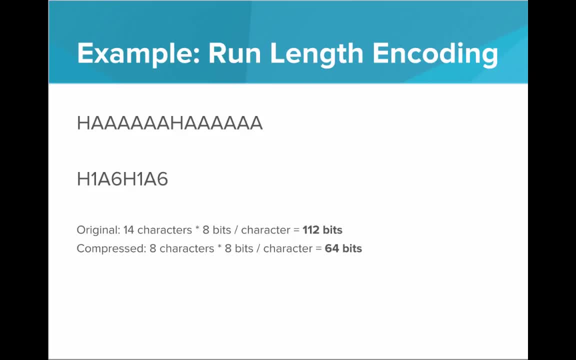 for example, if we take the run length encoding example, The original was 112 bits and the compressed was 64 bits. So to calculate the space savings we simply do 1 minus 64, the compressed size divided by 112, the original size multiply. 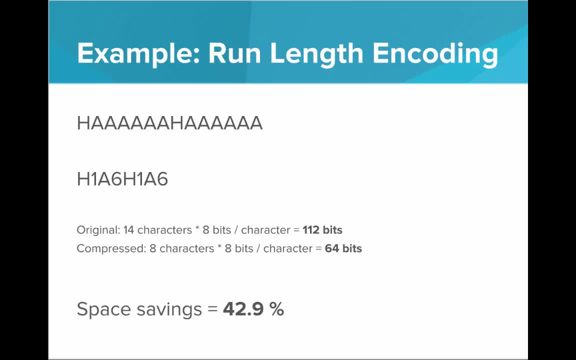 that by 100. And we see that we actually have a 42.9% space savings. The compressed data is 42.9% smaller than the original. That's pretty good. that's saving a lot of space. Now there are a lot of compression algorithms. Run length encoding is just a single example. 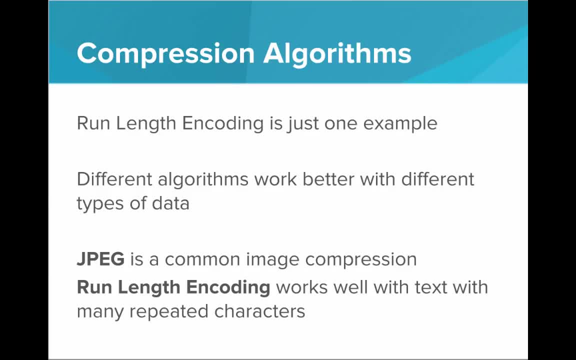 This is a huge field of computer science- is finding better and better algorithms to make data smaller. There's a lot of algorithms to choose from, And it turns out different algorithms work better with different types of data. For example, JPEG is a common image. 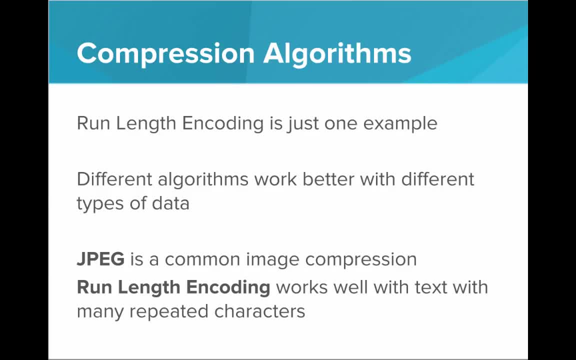 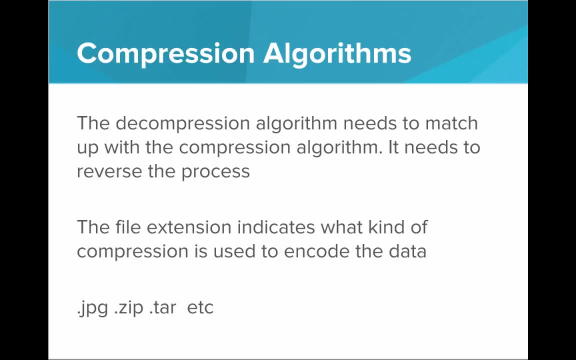 compression algorithm, whereas run length encoding works really well with text that has many repeated characters. Now, one important thing is that the decompression algorithm used needs to match up with the compression algorithm used. It needs to reverse that process. So the way we keep track of this, the way we keep track of which algorithms we're using, 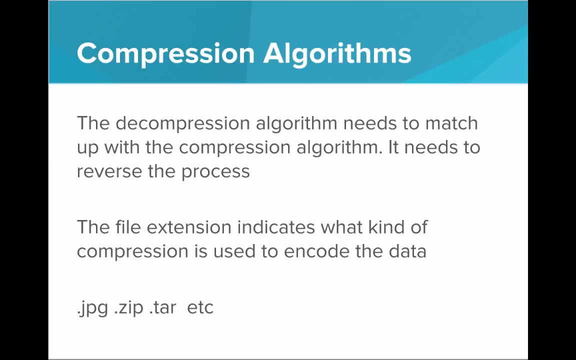 on which data is with file extensions. So a given file extension tells the computer what algorithm to use to decompress the data. So jpeg uses the JPEG compression algorithm. So when your computer sees a jpeg, it knows that that file was compressed with the JPEG algorithm, so it will need to decompress that. 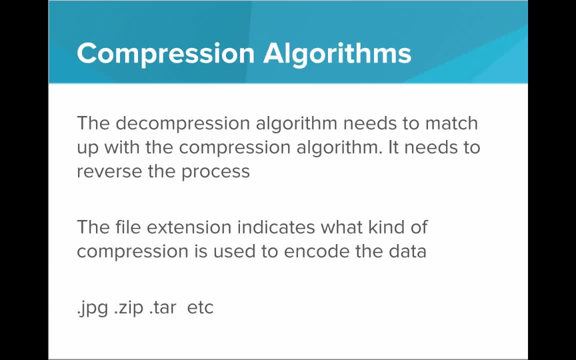 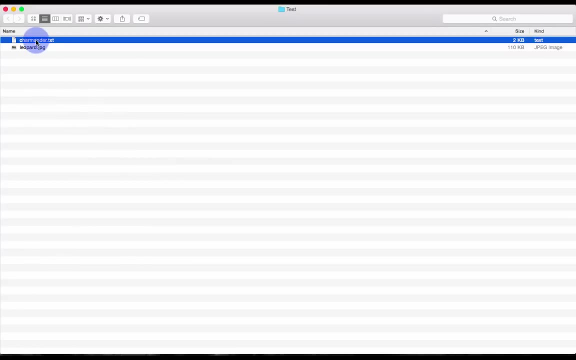 file with the same JPEG algorithm, So jpeg, zip, tar. these are all examples of different compression algorithms that produce different file extensions. So let's see an example of what these file extensions look like on a real computer. So I have a folder with two simple files. If I open up this Charmandertxt file, I see: